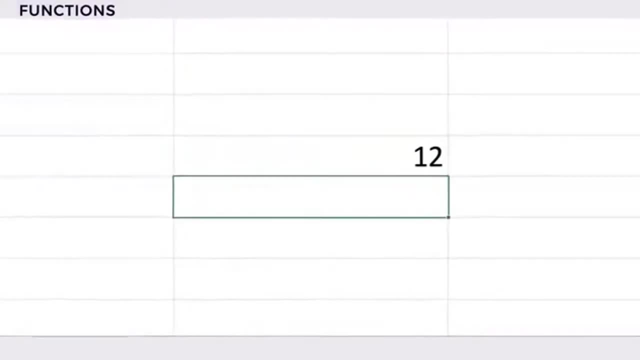 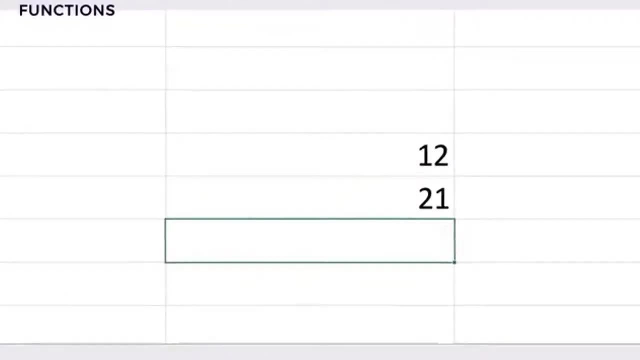 5 and 7.. Here, sum is a function that takes a list of inputs and it adds them. The function's function is to add numbers. Hash functions are the same, but they don't output a simple sum. They output what is called a hash, which looks something like this: It looks like random text. 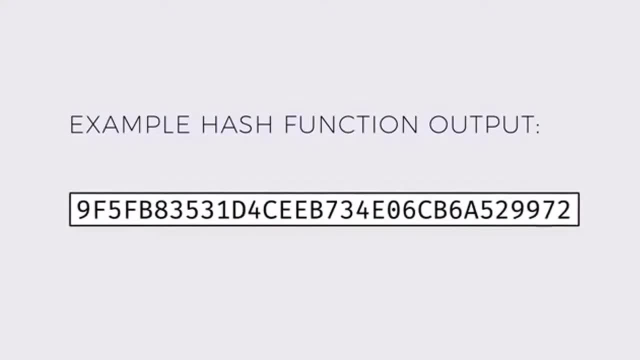 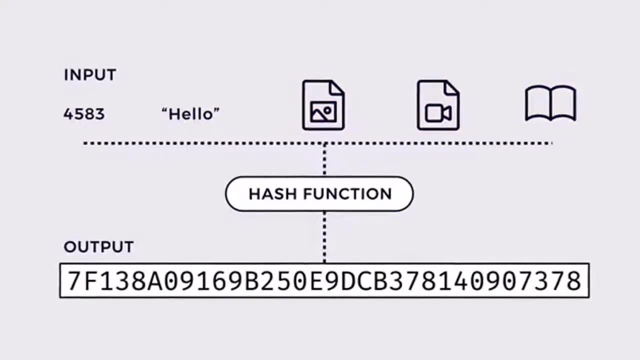 but it is not. A hash function takes as its input just about any kind of digital data- Numbers, text, images, videos, ebooks- of any size- and output what seems like a long string of random characters. This is a function that takes a list of inputs and it adds them. The function: takes a list of inputs and it adds them. The function's function is to add numbers. Hash functions take as its input just about any kind of digital data- Numbers, text, images, ebooks of any size- and output what seems like a long string of random characters. It can be also called a digest. 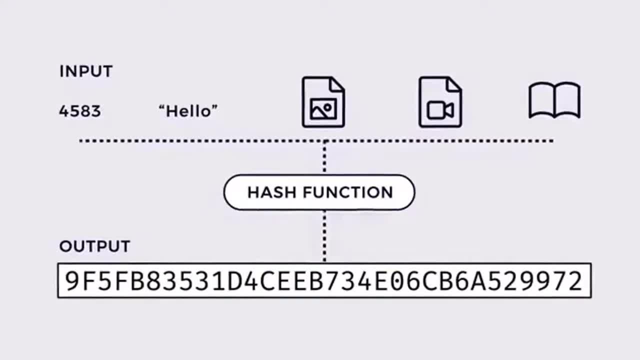 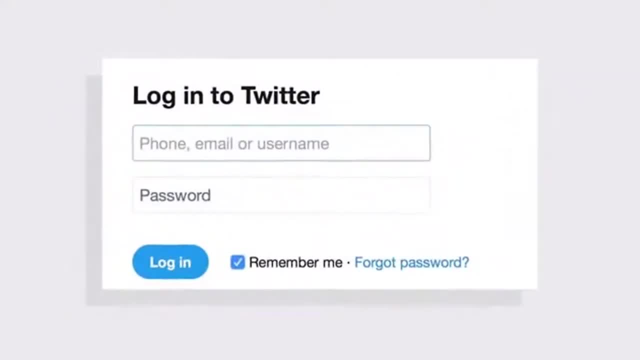 but we will just call it a hash. So what is big deal with that? How is that useful? Well, the properties of cryptographic hash functions give them some very interesting uses. For example, think of when you log into an app or a website, When you enter your password. a comparison: 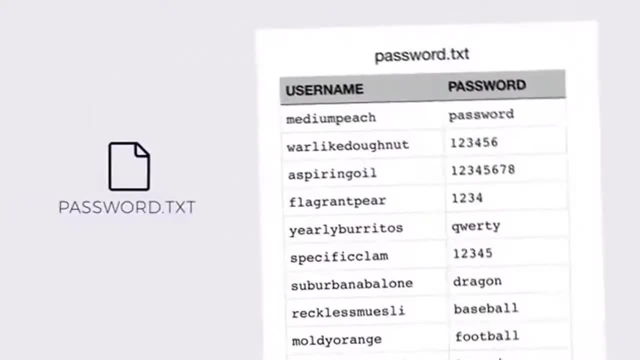 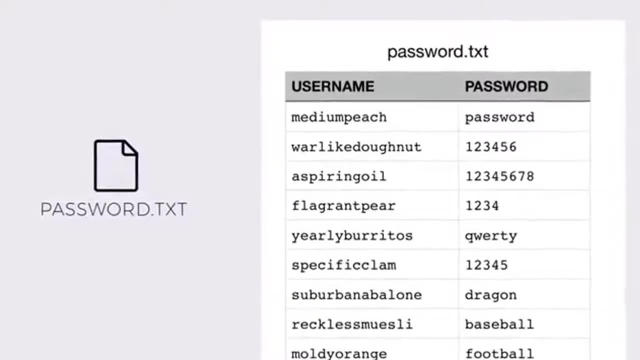 happens behind the scenes to see if the password you entered matches the password stored for your account. But your password isn't just stored in some text file on the server. That would make it way too easy to hack If an intruder got access to the password file. 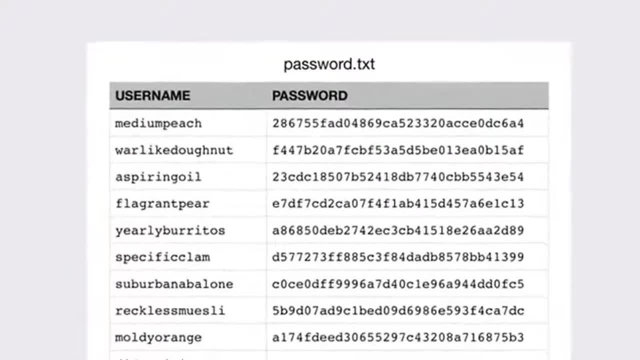 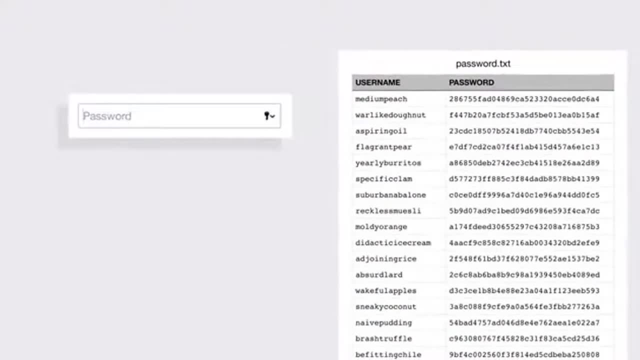 they would have all the user passwords for the entire system. So what you can do here is use a hash function Instead of storing your password. a hash of your password can be created and that is stored. Now the details are: when you go to login, the password you type is hashed with the same. 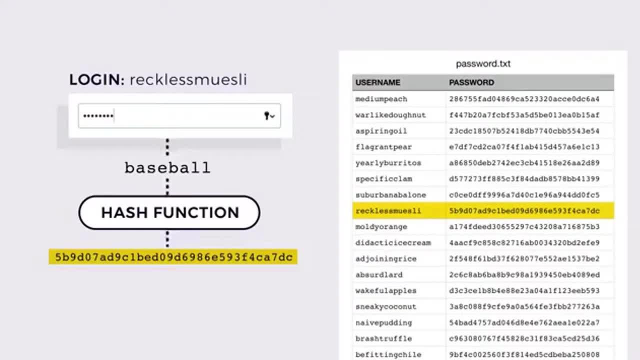 function that was used when you originally created it. And then the two are compared: Your actual password isn't stored anywhere. Your actual password isn't stored anywhere. Now you might be thinking, wait a minute, couldn't someone just take the hash password and reverse? 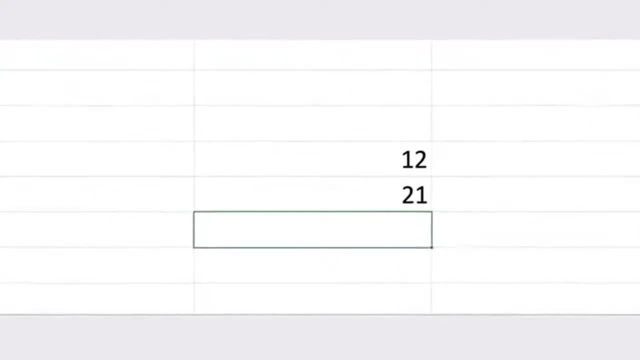 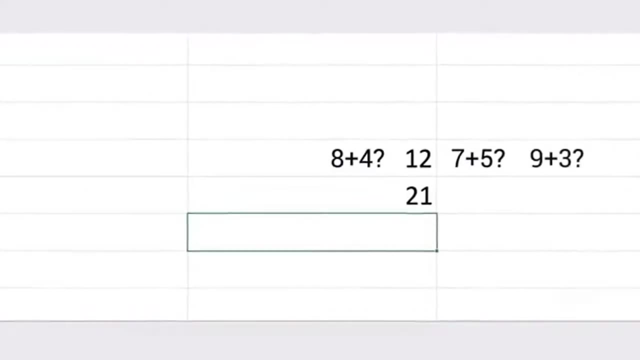 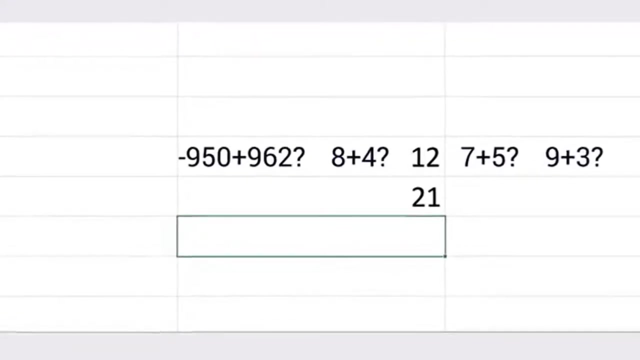 engineer the hash function to recover my password? The simple answer is no, In the same way that if you knew that 12 was the final result of the sum function in a spreadsheet, you wouldn't know if I summed 7 and 5 or 4 and 8 and so on. Except the cryptographic hash functions, the math 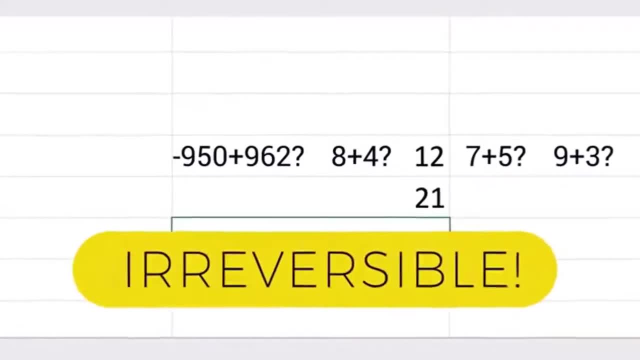 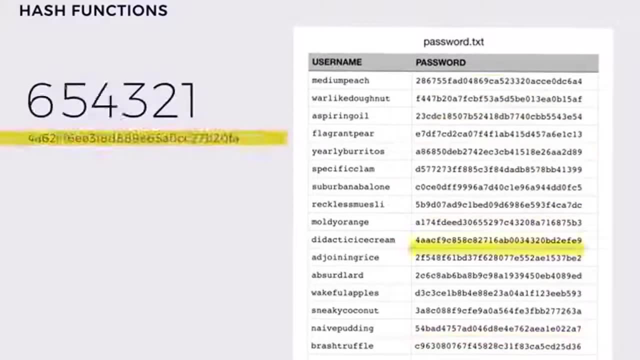 is far more complicated, But an extremely important property of these hash functions, one that makes them so useful, is the cryptographic hash function. The cryptographic hash function is the one that makes them so useful is their irreversibility. If hackers manage to get a. 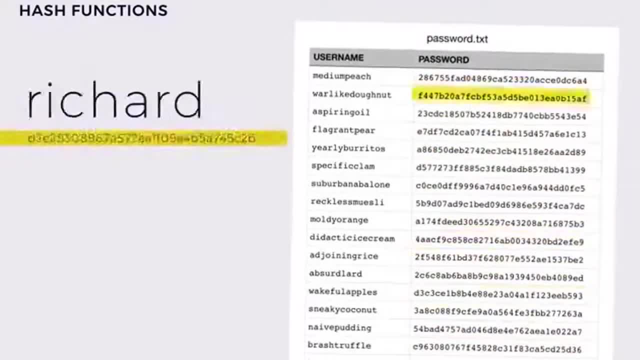 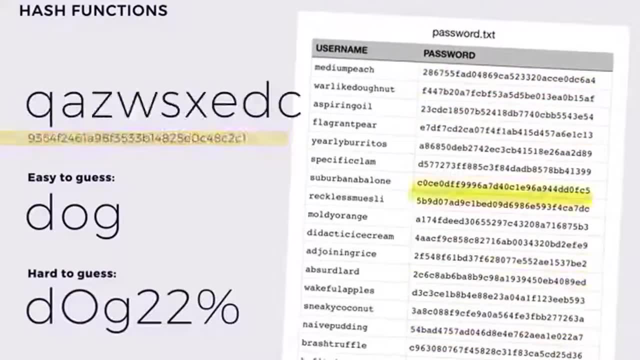 password file. the only way they can guess your password is to do what is called a dictionary attack, where they hash common words, phrases and variations to see if they can find matches. So if your password is dog, they will be able to find it pretty quickly. This is why, when you 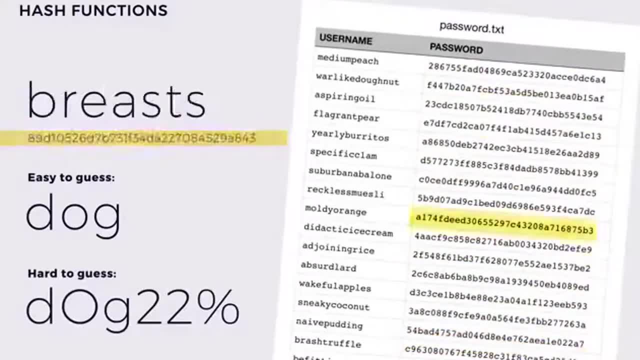 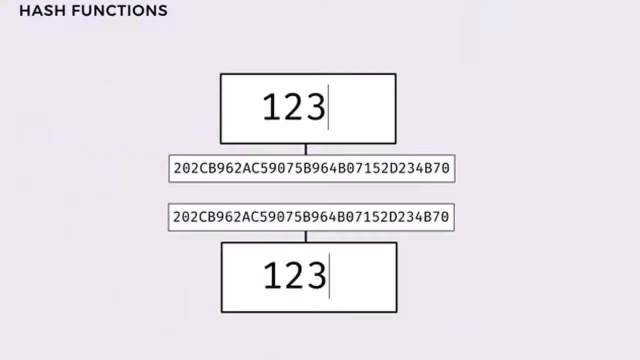 create passwords. these days, you are asked to add letters, capitalizations, numbers and symbols, because it is far less likely that hackers will think to hash something like dog. 22%, which makes your password more secure. If your password is 1234 and mine is 1235,, look at the. 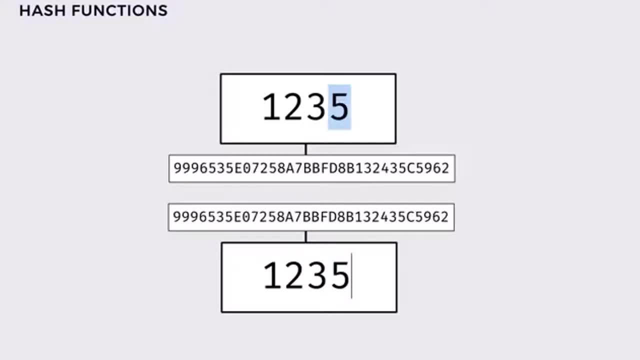 hashes. They are completely different, Even though our passwords differ by just one character. not only are hashes irreversible, but even inputs that are very similar or close to each other end up completely different. You can see that as I type here, the hash keeps changing because the text 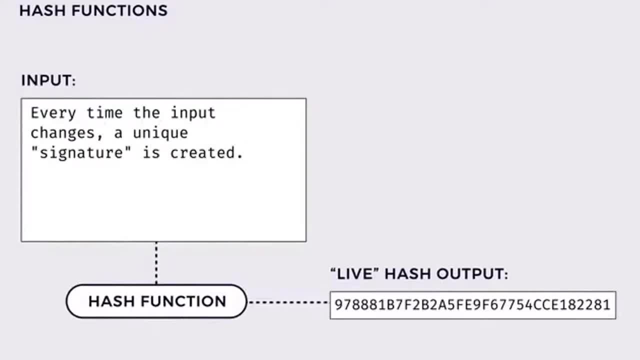 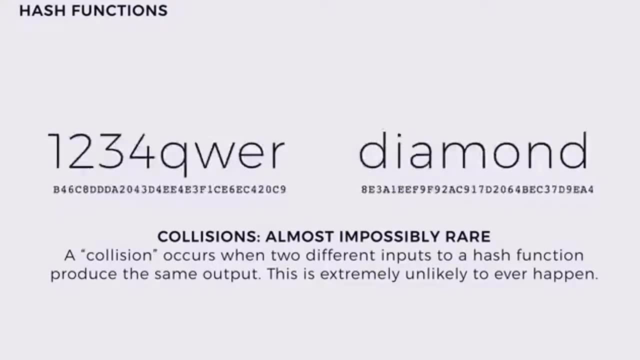 input is changing, And if I change just one letter you get a totally different hash. You can think of it as like a unique signature of a given input. Another property of these hash functions is that the chances of one password generating the same hash or another- something called a collision. 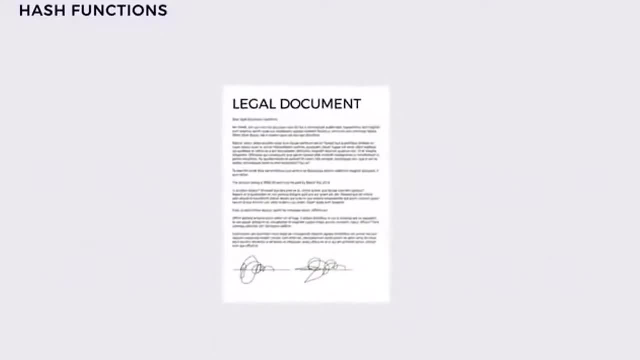 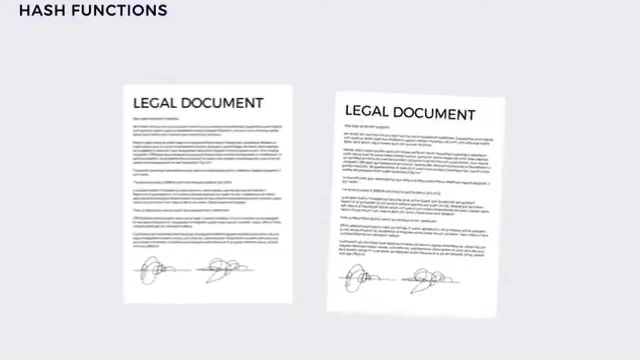 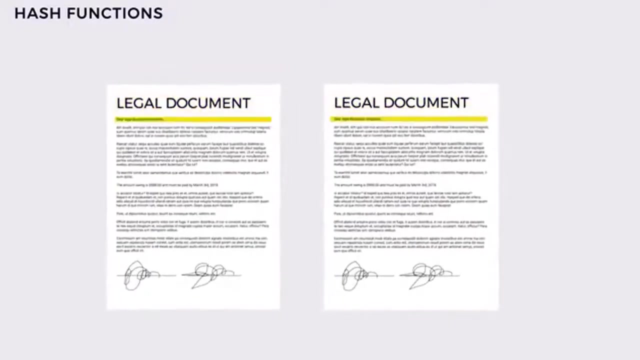 are so unlikely as to be, practically speaking, impossible. Let's look at another example. Imagine you created a legal document and it was sent for review. It was sent back to you again, approved without changes. How could you tell that the document was not any way altered? Well, you could. 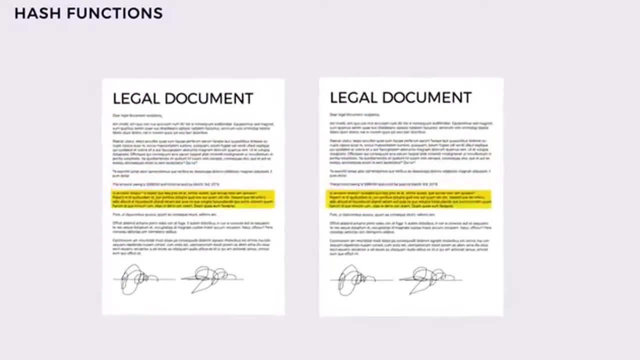 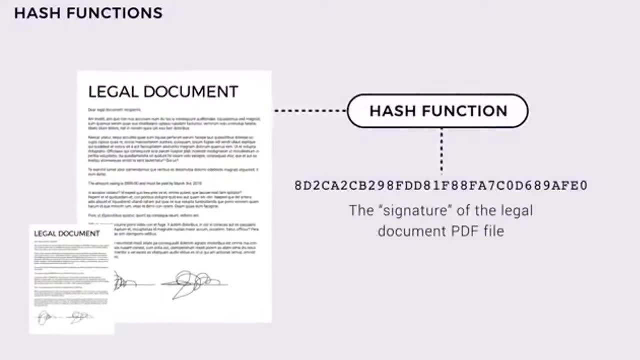 read the document line by line and ensure it matches the original. Or maybe you could take a hash of the original document and compare it to a hash of the received document, Because the hash function outputs a unique fingerprint of its input data. you can be assured that if the document was 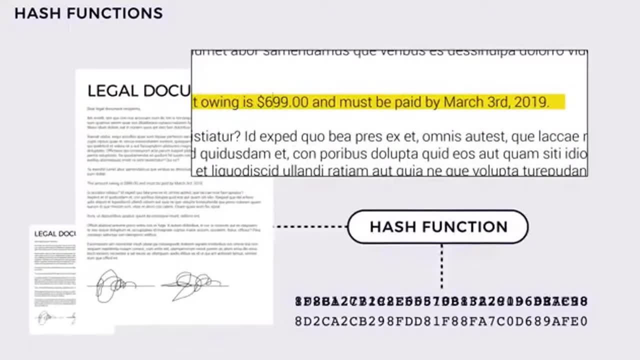 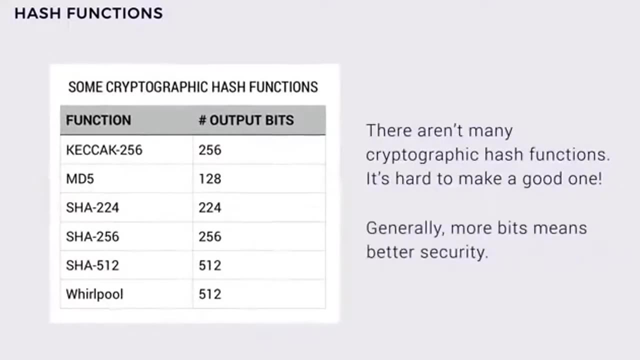 altered, the hashes wouldn't match And that, if the hashes are matching, the documents are identical. Different cryptographic hash functions have different names and often have associated numbers related to the length of their output. One common hash function is SHA-128,, which stands for the standard hashing algorithm and its output.